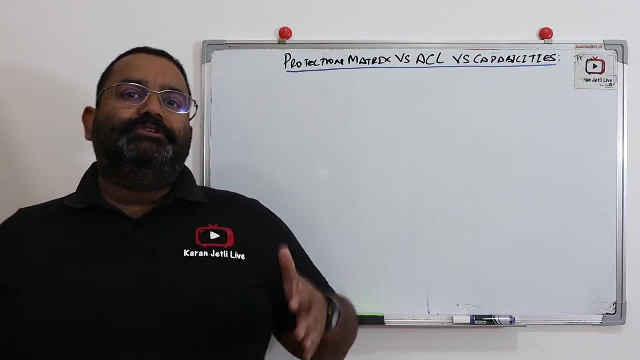 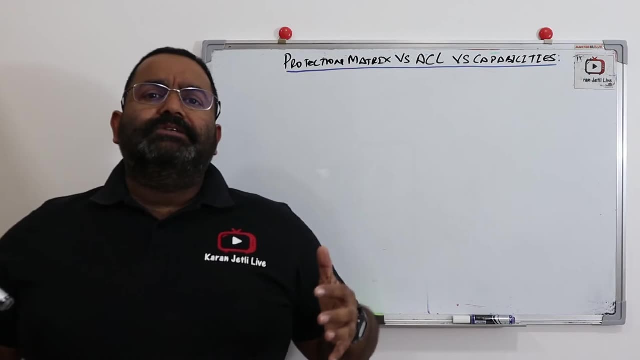 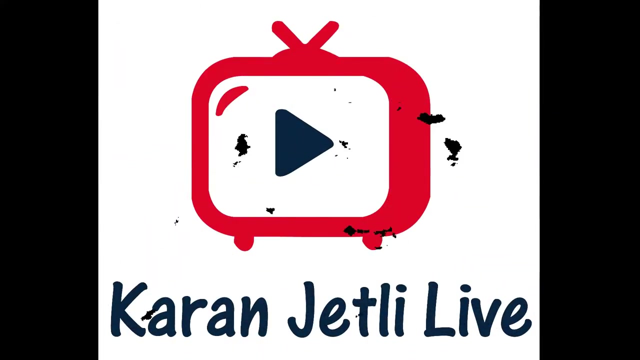 Hi guys, welcome to my channel. And today, in this video, we are going to discuss protection metrics versus ACL lists, versus capabilities in operating system security. So, guys, for the whole video, all of you, stay tuned. So, guys, the first thing which comes is the protection metrics. Okay, So to give you an, 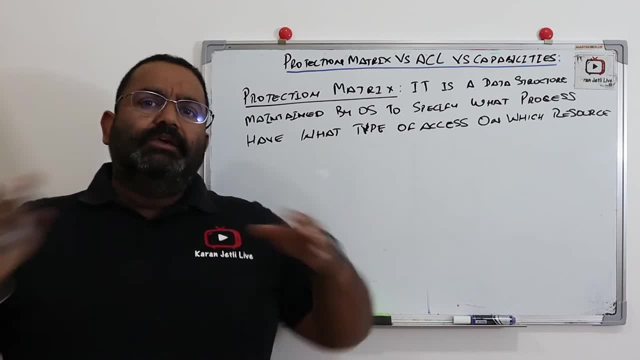 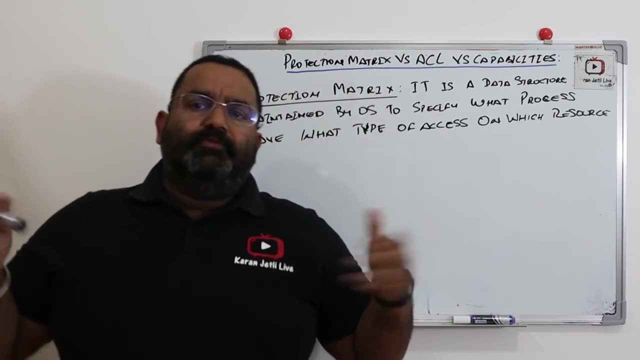 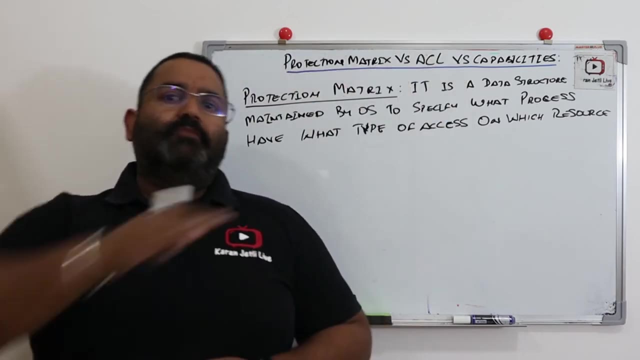 idea what is a protection metrics. Protection metrics is basically a metrics which is maintained by the operating system. Okay, So it is a data structure. Why I'm saying it is a data structure? So metrics is also a type of a data structure in which the data is stored in forms of rows and 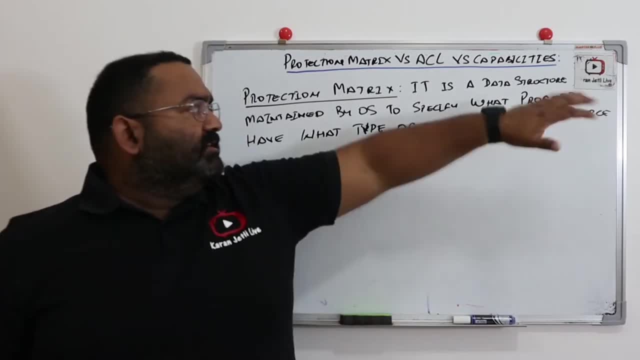 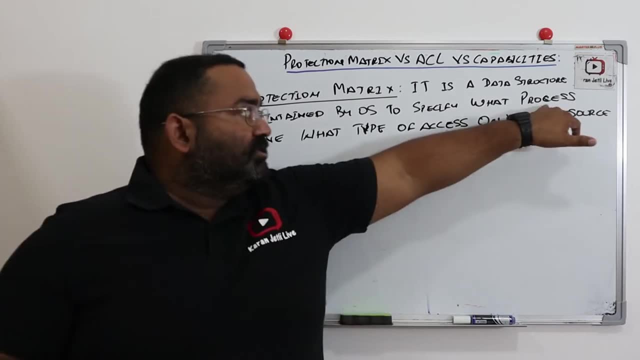 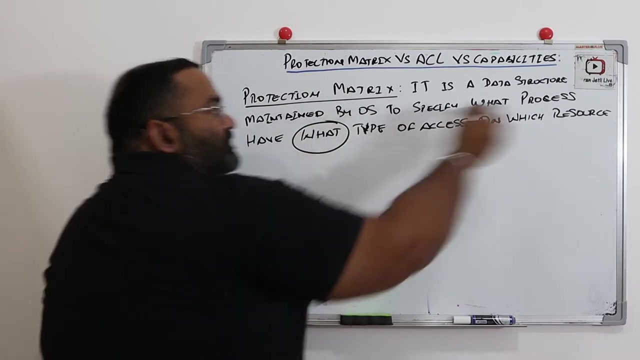 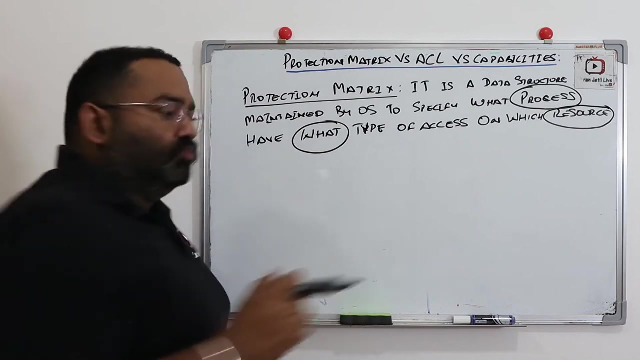 columns. Okay, So what is a protection metrics? It is a data structure which is maintained by the operating system, which specifies which process, which specifies which process has what type of access, Which process has what type of access, Which process has what type of access on which resource, on which resource. 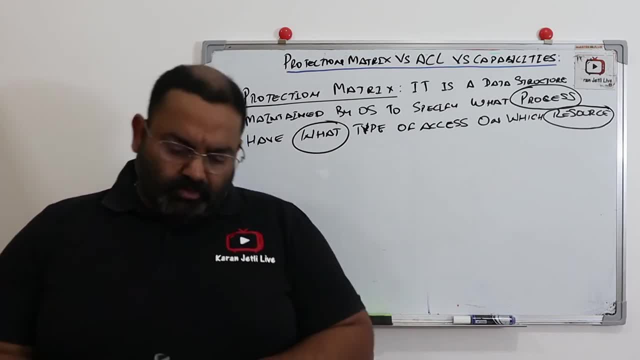 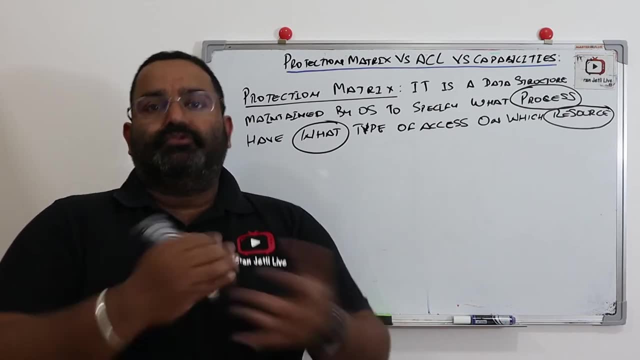 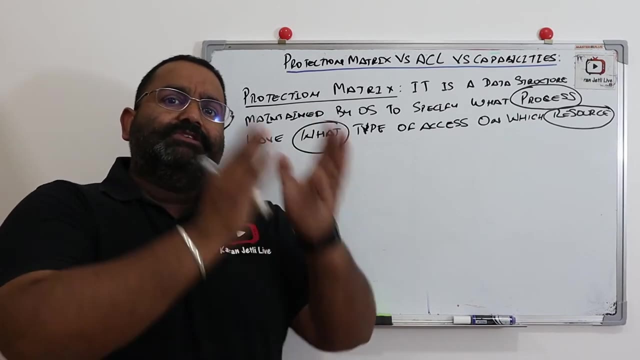 Now, guys, if you know how security works. how security works means one of the most important aspect of security is access control. is access control? What do I mean by access control? It means only the processes which are authorized to access some resources, only those. 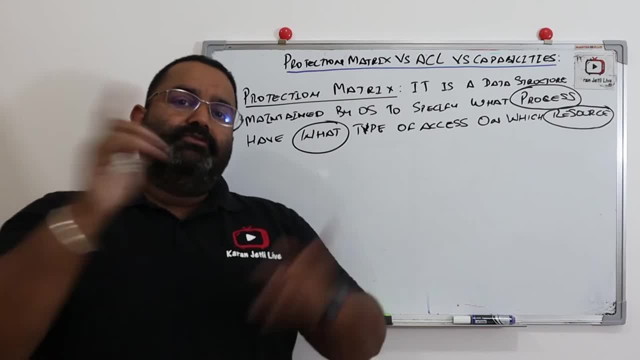 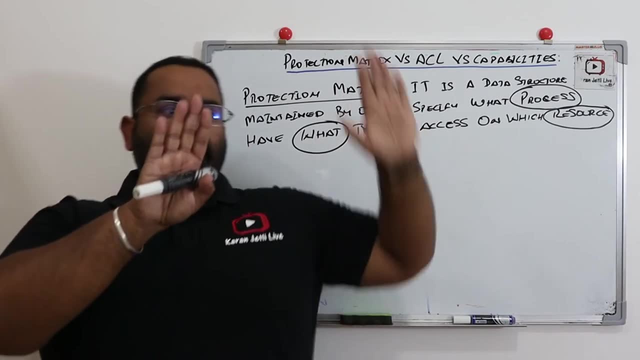 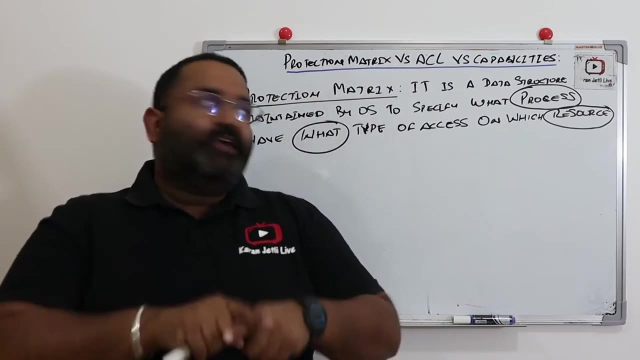 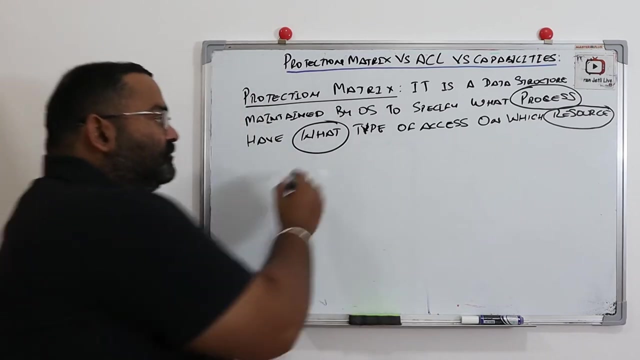 processes should access those resources, not any other processes. Okay, So what is access control? I have a process, I have a resource. Okay, Which process can have what type of access on this resource is specified in a matrix called as protection metrics. For example, I have a process P1.. I have a process P1.. It has a resource R1 and 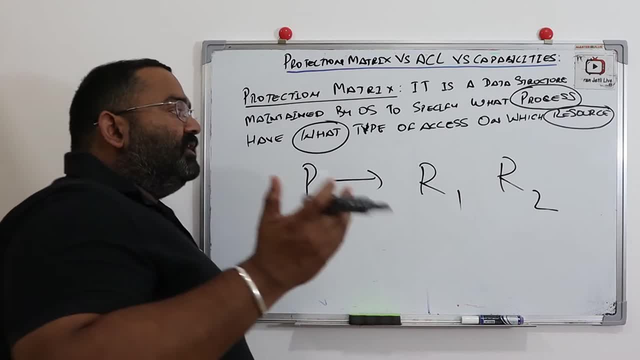 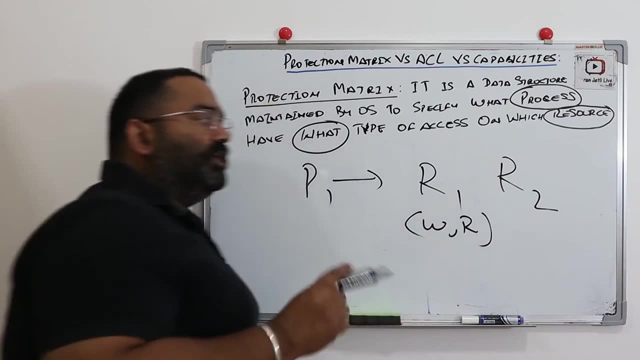 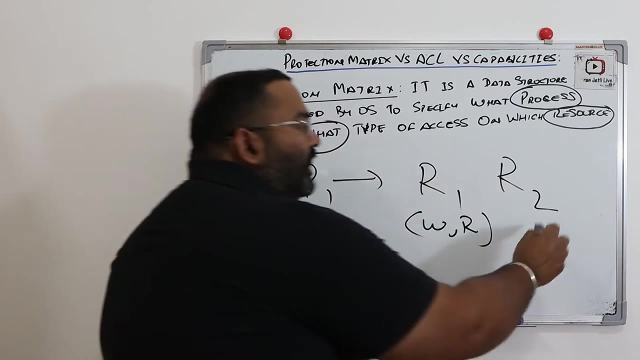 Okay, so what type of access P1 can have on the source R1. We can say P1 can rewrite and P1 can do read operation on this resource. Okay, what type of access P1 has on R2? I can say, on R2 P1 can do only the read operation. 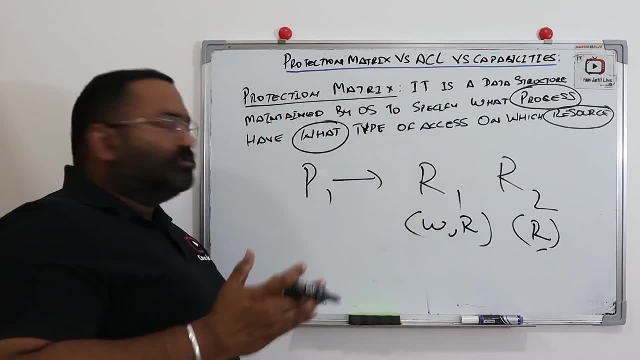 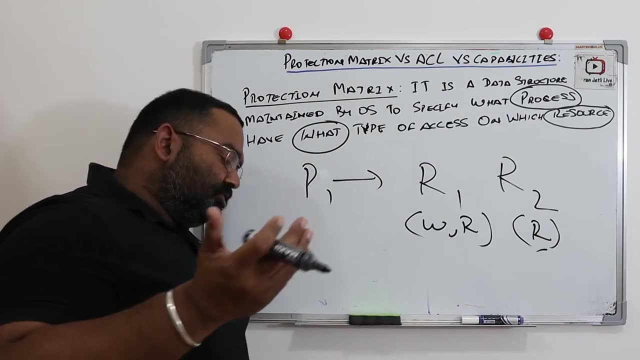 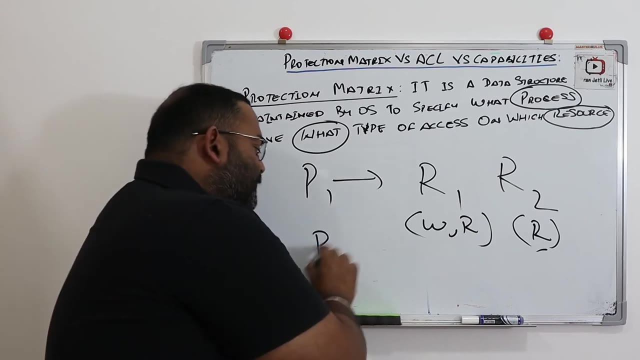 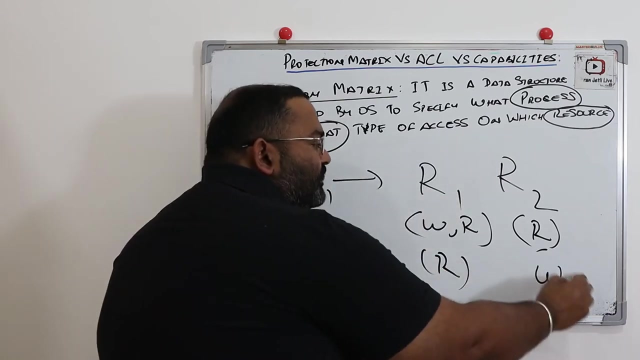 Okay. so when I maintain a data structure which specifies all the processes, all the resources and what type of access the resources, the processes, have on those resources, We call it as protection matrix. For example, we have another process, P2.. It has only read access on R1 and it has only read and it has read and write access on R2.. 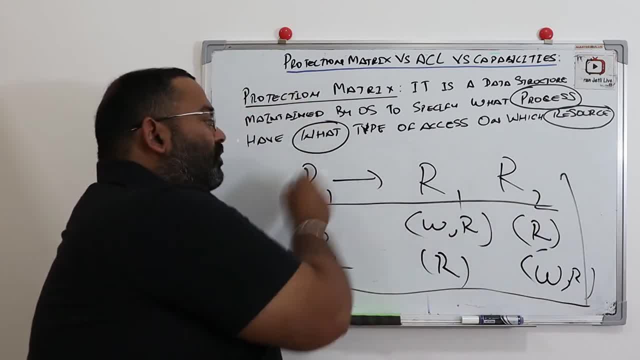 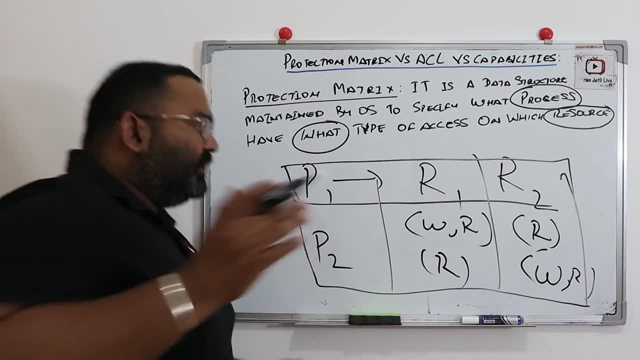 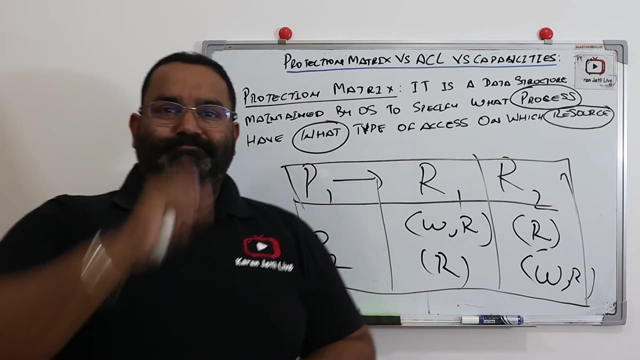 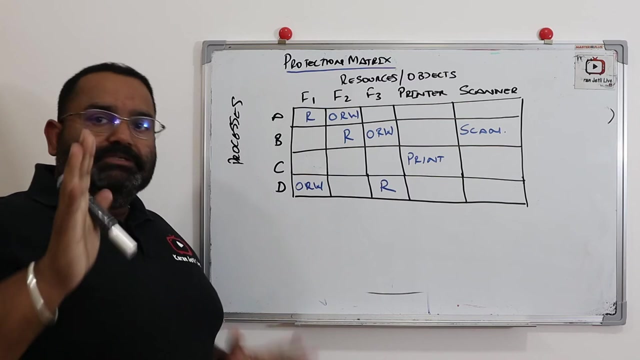 Okay. so when I maintain, Then in the form of our matrix, So what do we call it? We call it as protection matrix. So, guys, in the next part of the video I will make a detailed protection matrix to make it more clear to you. Now, guys, if you look at this, this is a typical protection matrix. Okay, so in this example, I'm showing you different resources. Okay, so, when we talk about resources in our computer systems, 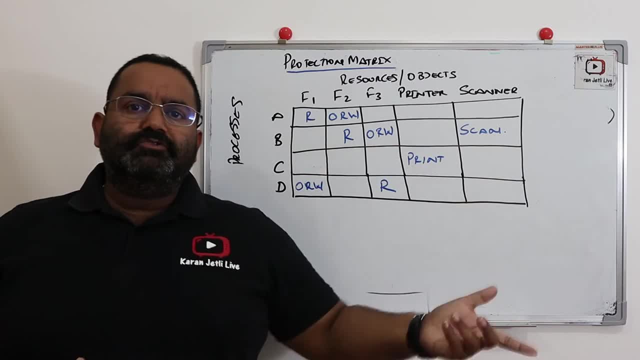 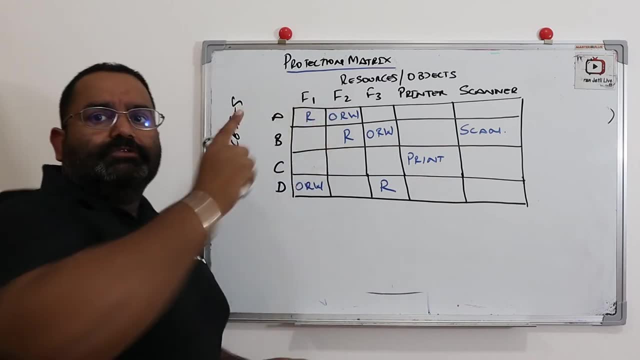 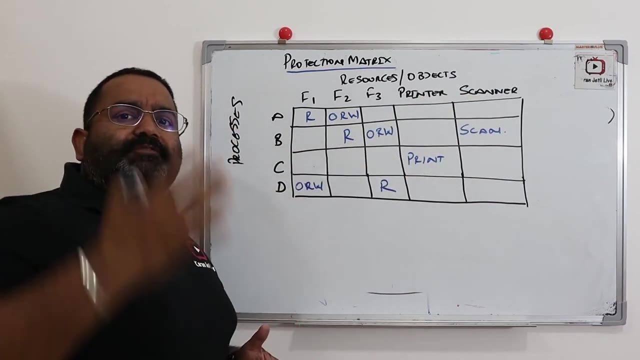 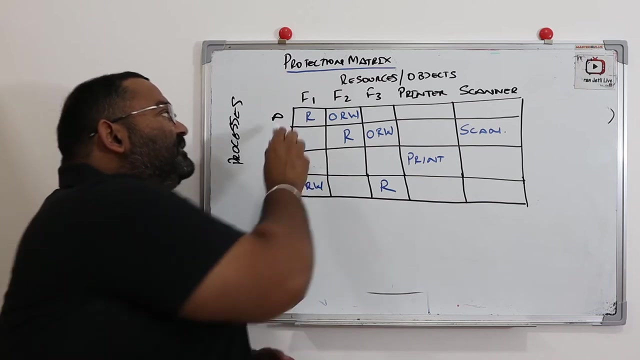 we are talking about resources in our computer systems. So when we talk about resources in our computer systems, we are talking about resources in our computer systems. We have many different types of resources. File is a resource. Your hardware resources are there, like printer, scanner and so on. Okay, so we have different resources. I have file 1, file 2,, file 3.. I have a printer as a resource. I have a scanner. So these are the different resources which are needed by different processes. So in this example, I have four processes, that is, A, B, C and D. Okay, now, if you study this matrix, you will come to know that there are four processes. 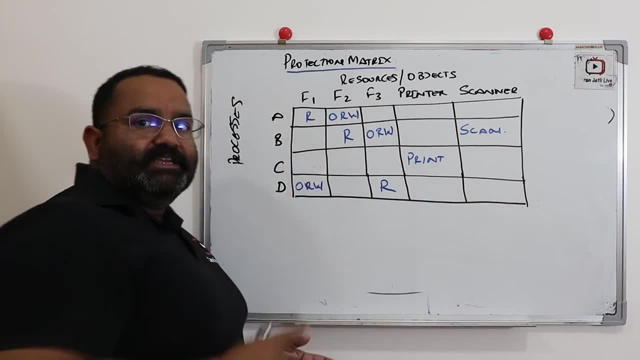 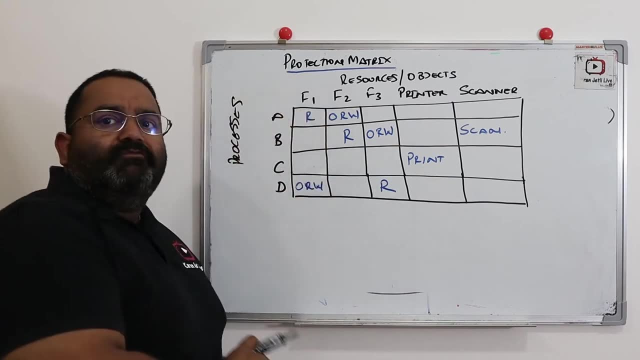 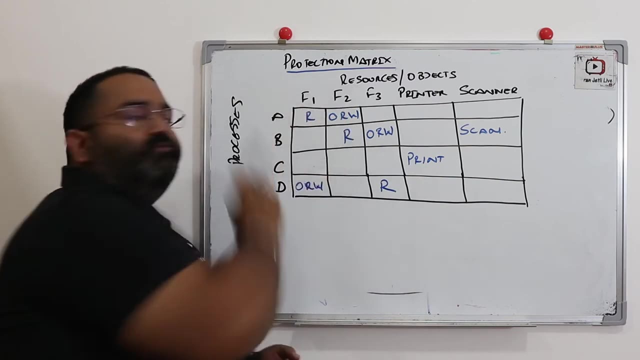 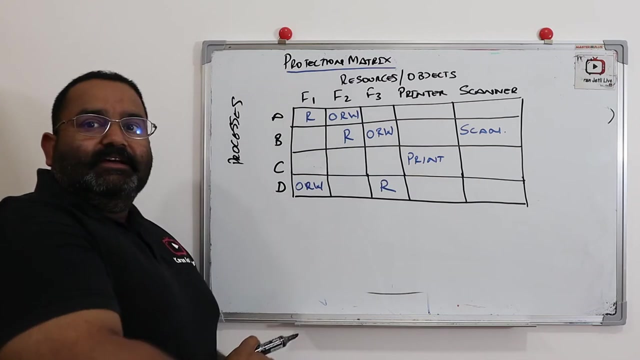 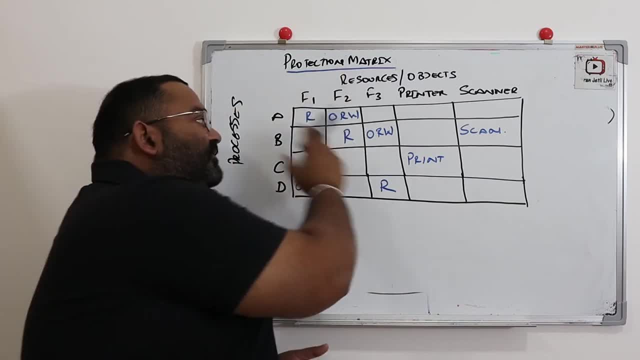 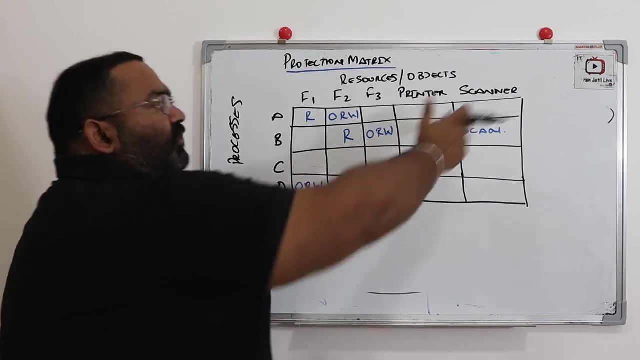 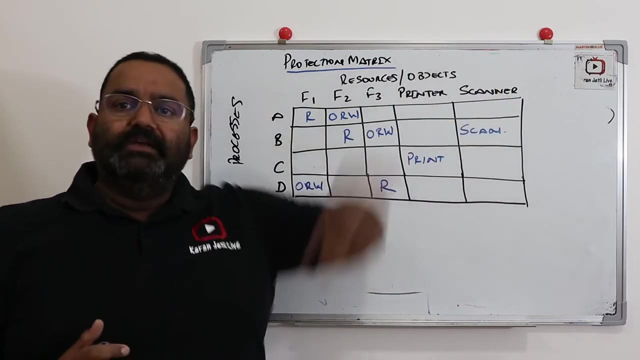 It has on file F2.. It can read the file And F3, it owns it. It can read it, It can write it, And so on. Okay, so what type of access it has on the scanner? it can use the scanner. It can scan the documents using this resource. 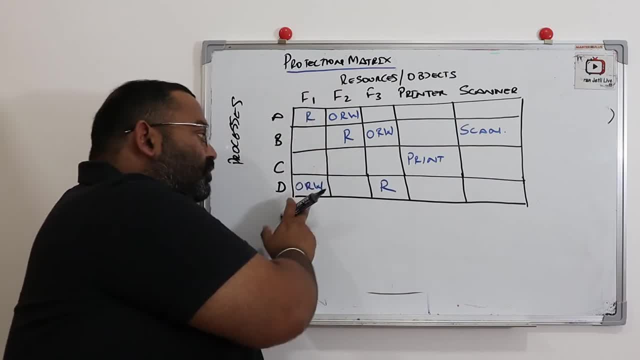 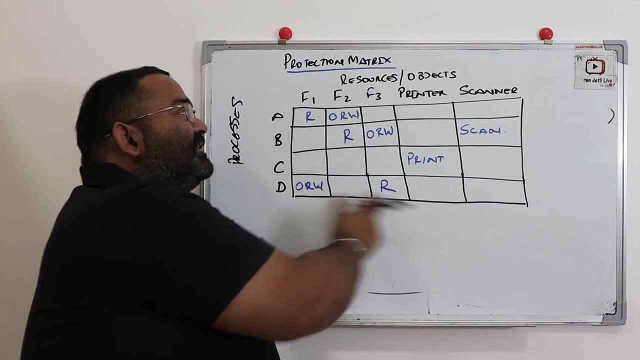 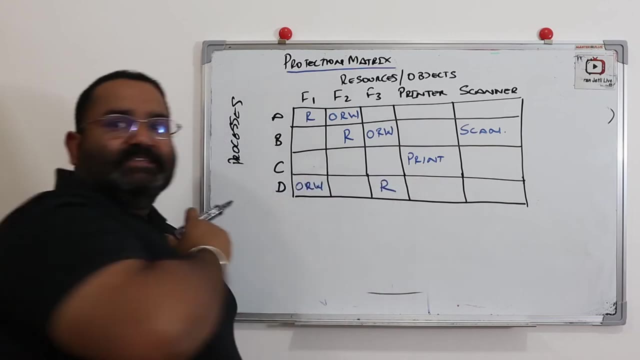 Similarly, I have process D, So it owns file F1. It can read on F1.. It can write on F1 and it can do only read on F3.. Okay, So here what we are specifying the type of accesses, Here what we are specifying all the resources and here what we are specifying all the processes. 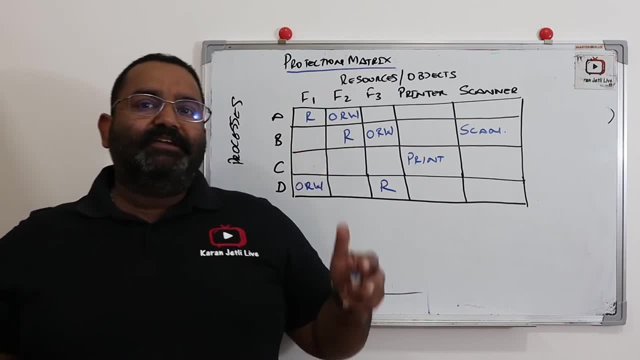 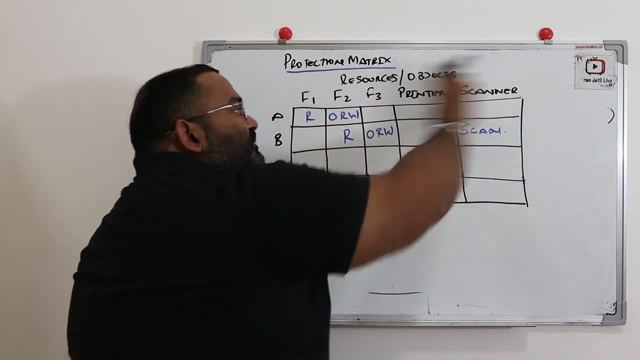 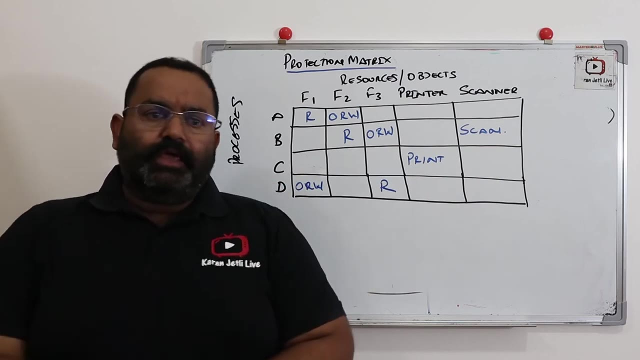 As I told you in the definition, the protection matrix. it specifies what type of access, what process has on which resource. Okay, So what do we call it? We call it as protection matrix, Okay. So, guys, I hope this is clear to you, Okay. 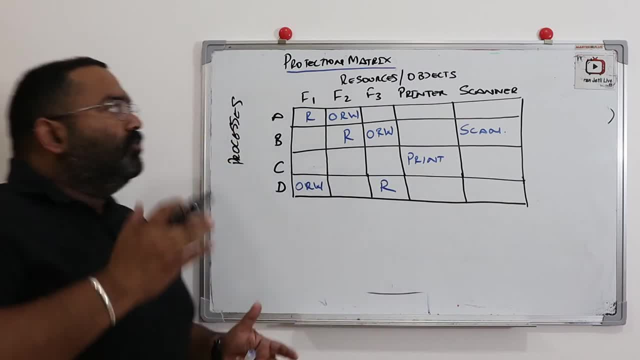 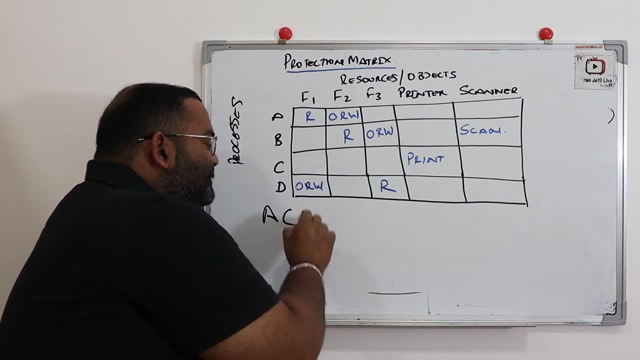 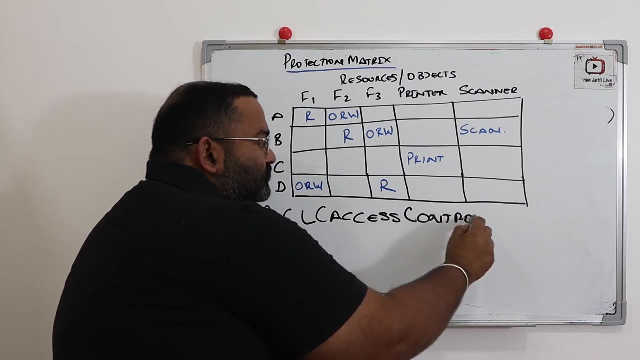 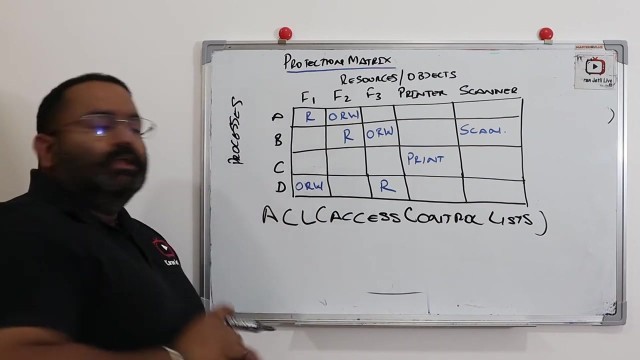 After this, the next thing which comes when we talk about protection matrix, with the protection matrix also another term called, we call it access. It is also known as ACL. What do we call it? Access control lists. Now, what is an ACL? So, before we discuss ACL, we will discuss an issue with the protection matrix. 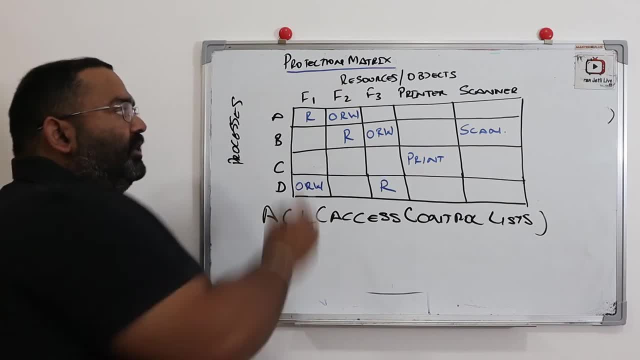 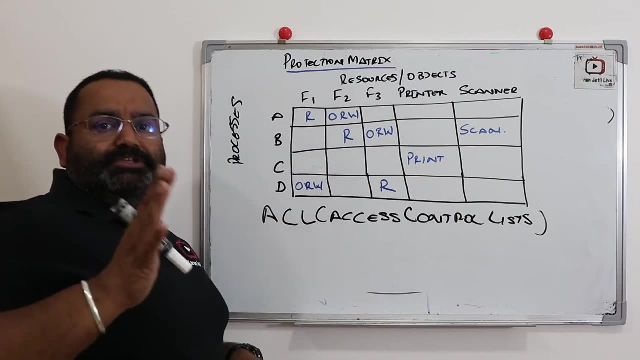 Now, guys, if you look at this matrix, okay, here, all the cells of this matrix, they are used, They store some information. Okay, So here, all the cells of this matrix, they are used, They store some information. So here, all the cells of this matrix, they are used, They store some information. 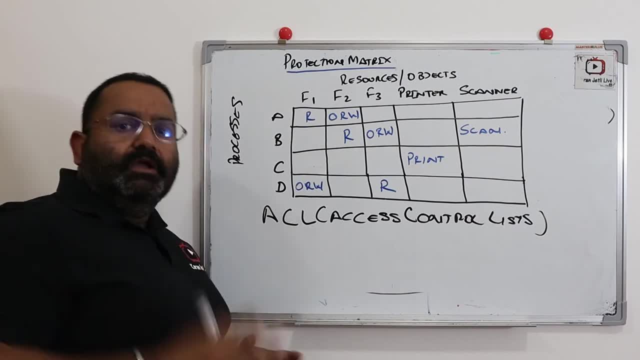 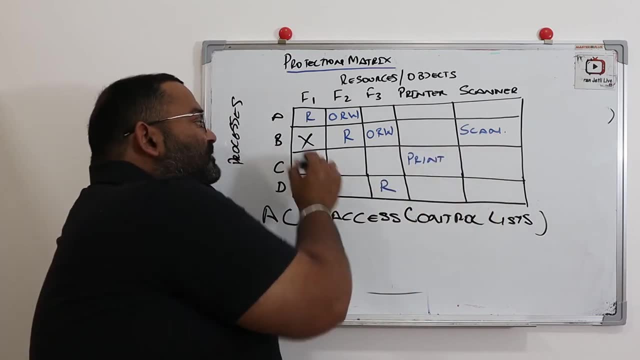 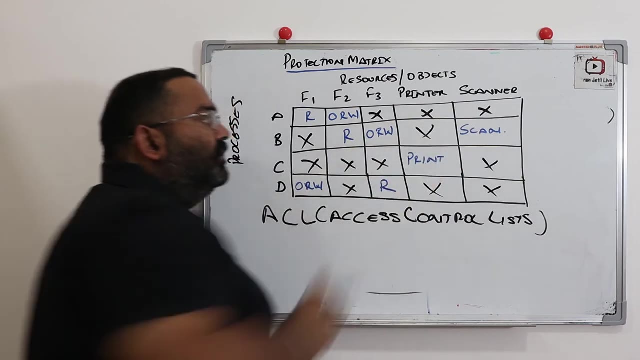 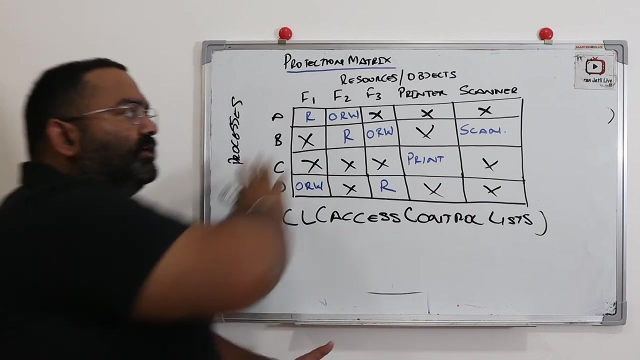 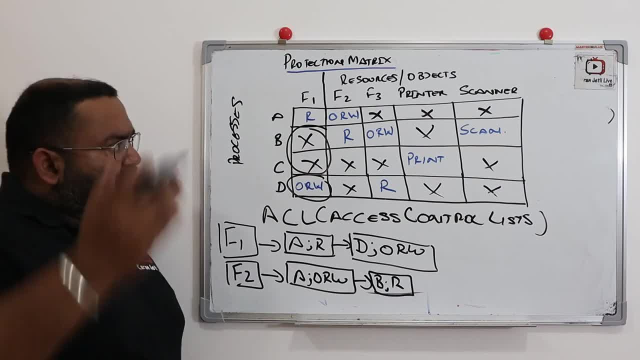 Okay, So here all the cells of this matrix. they are used, They store some information. Okay, So here all the cells of this matrix. they are used, They store some information, And that's it. Similarly, let us go to file F3.. I hope you can see it. So what it can do. F3,. 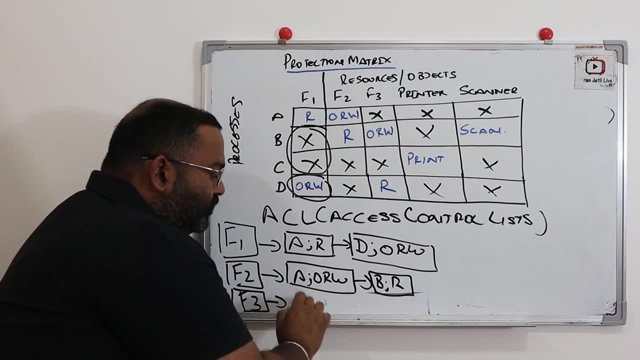 what it can do on A, Nothing, So we leave it. What it can do on B, What it can do on B, It owns it, reads it, writes it. What it can do on D, What it can do on D, It can do a. 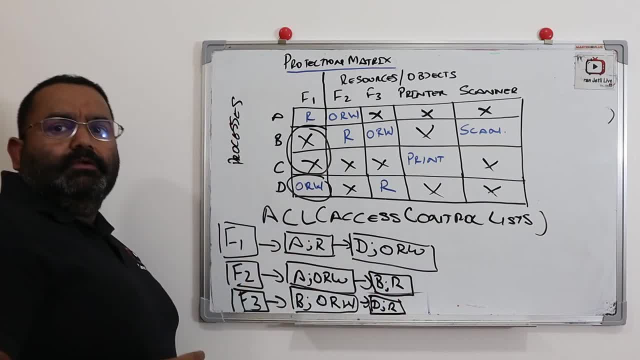 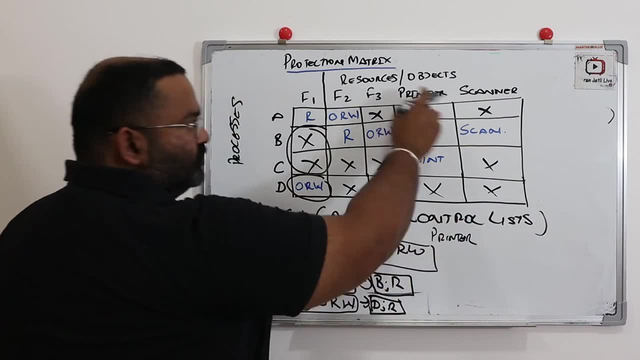 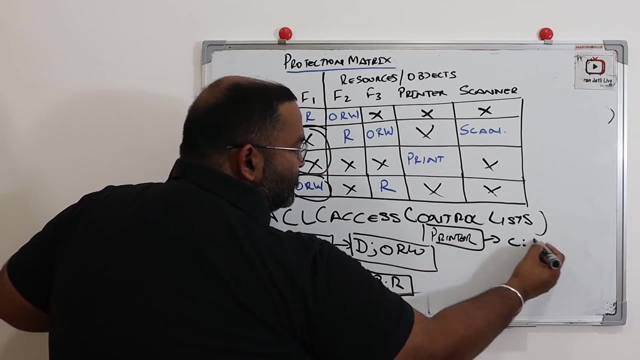 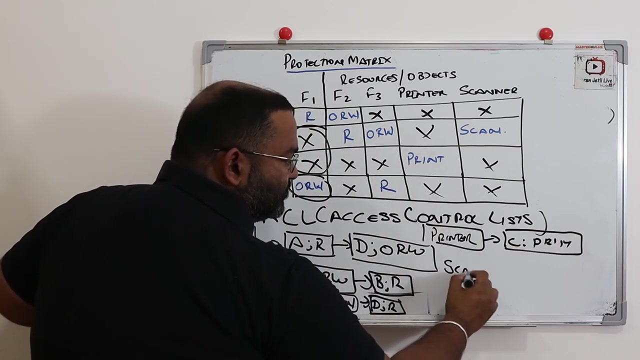 write operation on D. Similarly, I can make one for the printer. So what printer, which process can to use the printer? Process C, C can do the print on it And that's it. Same for the scanner. Okay, So which process can use the scanner? 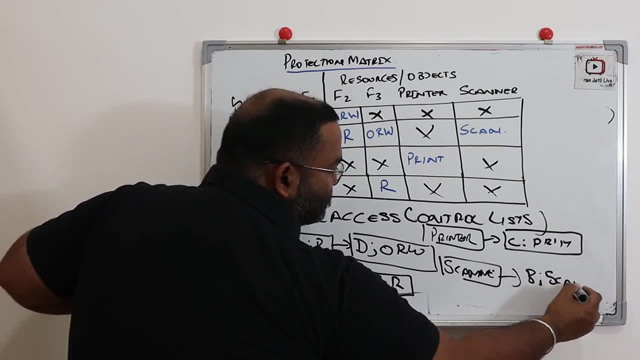 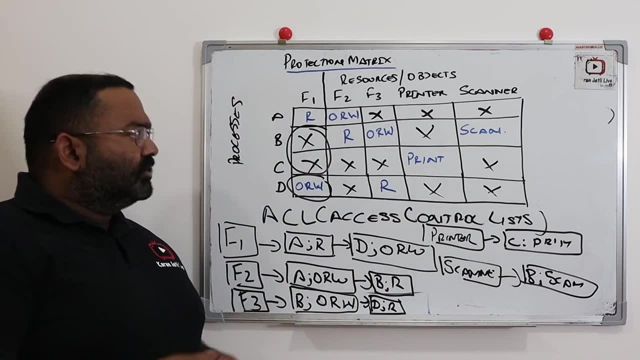 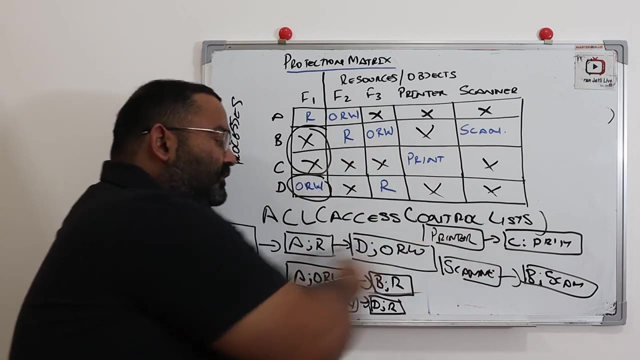 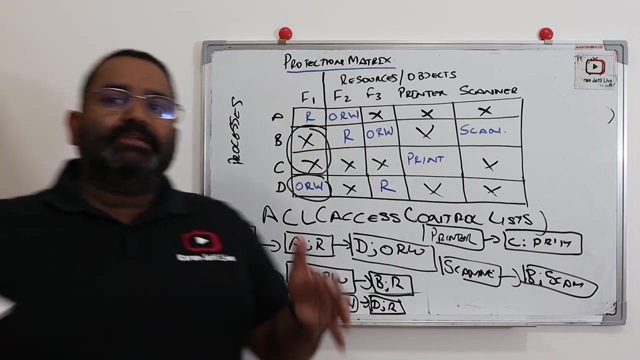 Process C, Process C, We can scan it, and so on. So what do we call it? We call it as access control list. So what is access control list? It is the implementation of production metrics in a form of a linked list. column wise, column wise. Okay. So, guys, after this, the next thing which comes: 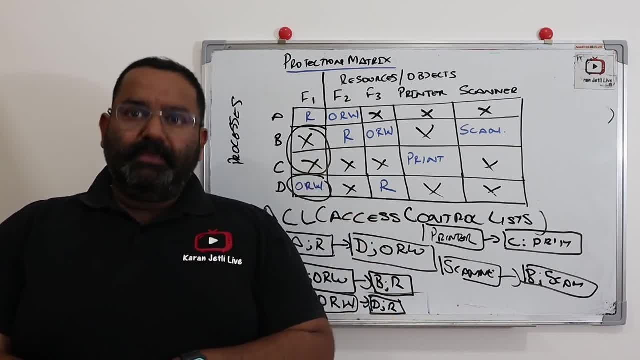 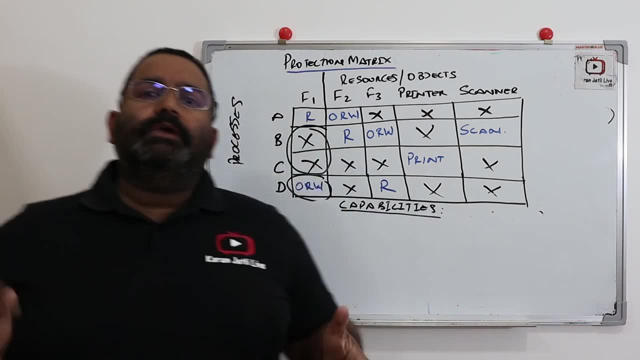 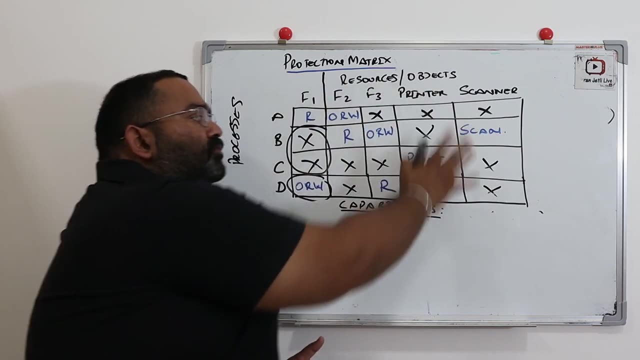 is called as capabilities. It's called as capabilities Now. we are going to discuss that. So, guys, when we talk about capabilities, now capability is also a linked list. like ACL, It is also a linked list using which we can implement the production metrics. 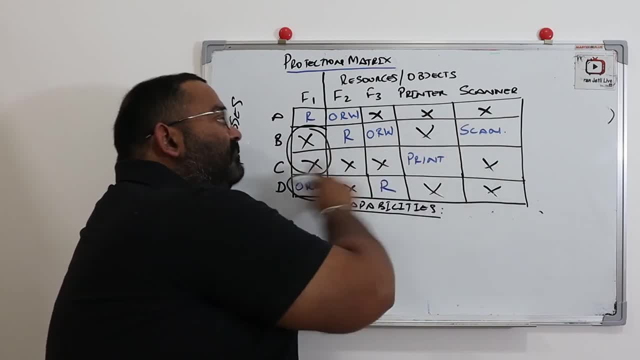 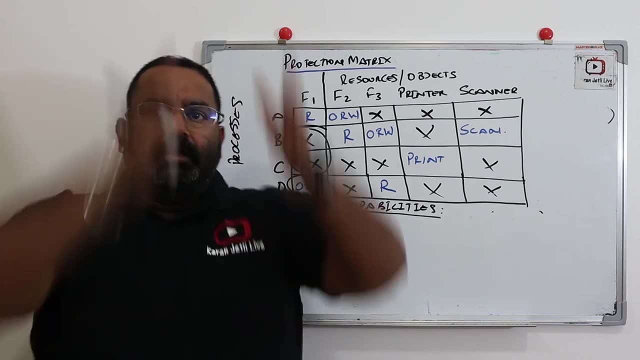 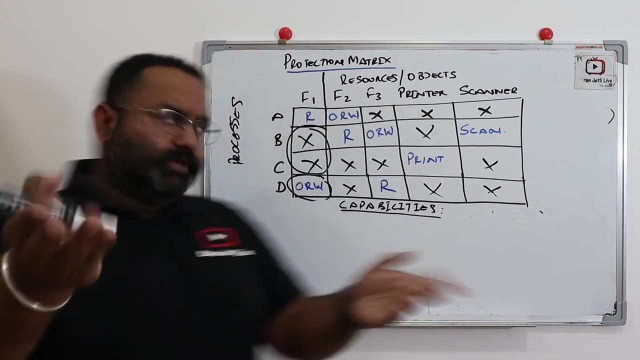 Okay. But here we will implement the production metrics on the linked list, row wise: Okay. ACL is implementation of the production metrics, column wise, and capabilities is the implementation of production metrics. Okay. And if you look at CCL, it is implementation of the processes, row wise: okay, Easy to make. 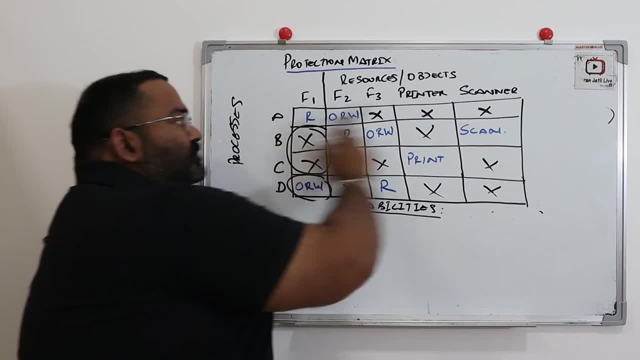 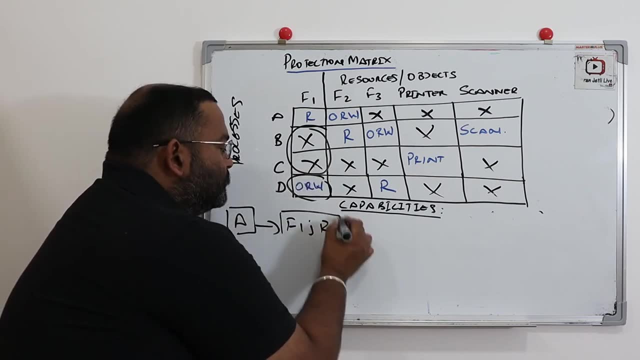 like ACL. So I have process A, I have process A, So lemme go row by row So process that I can file 1.. What it can do: It can do a read operation process A on file 2, what? 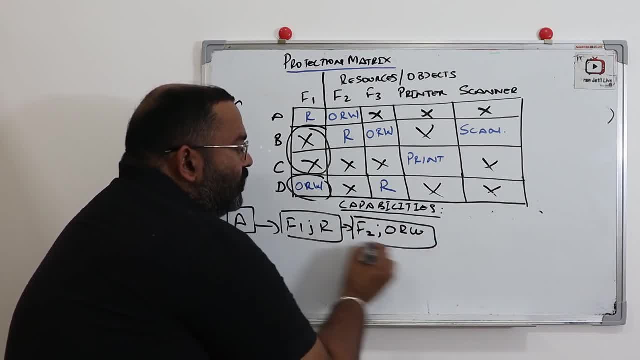 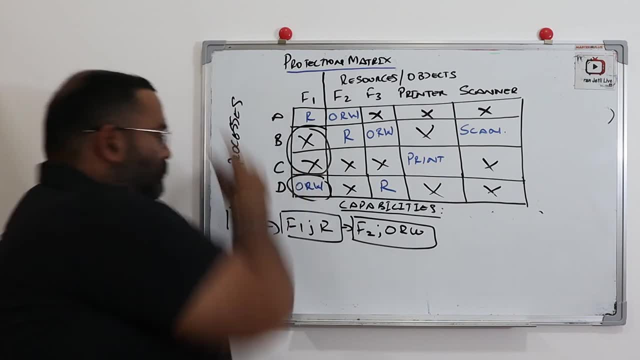 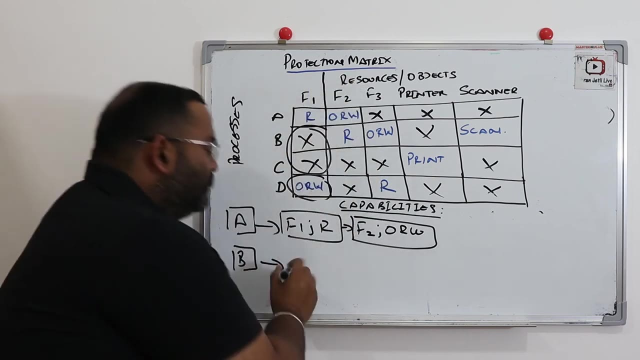 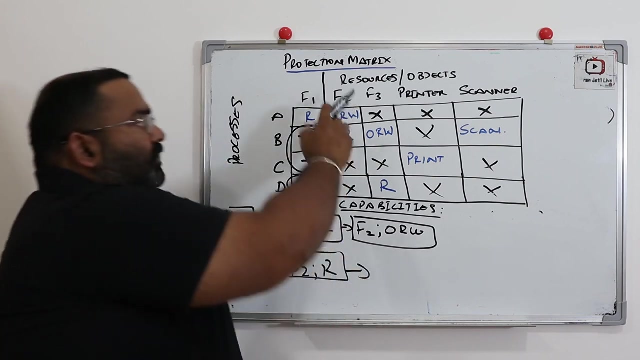 it can do, It owns it. it can do read, it can do write, and that's it. it row wise. now let us go to this process B. so process B. so on F1, it does not do anything on F2, what it can do on F2, it can do a read operation. then go to 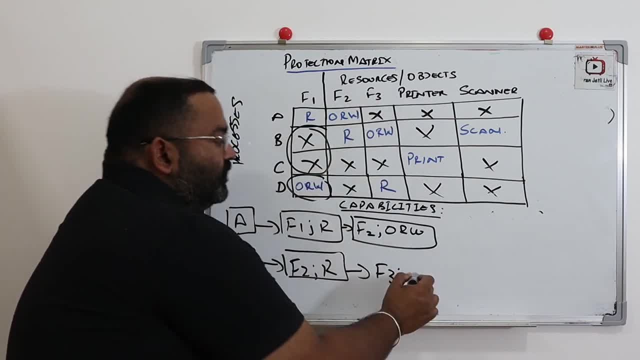 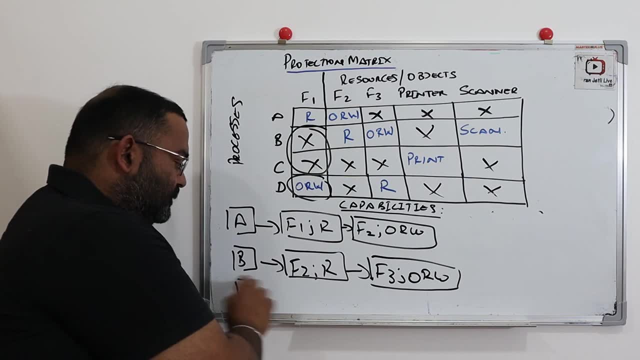 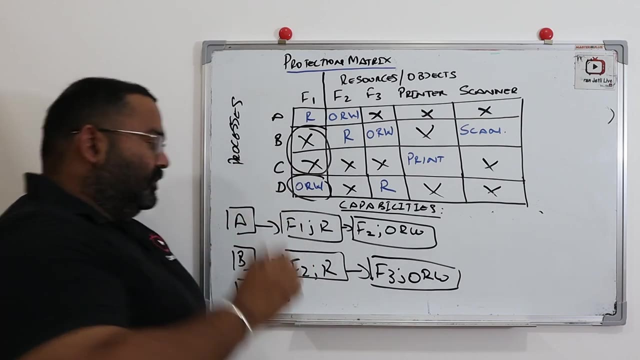 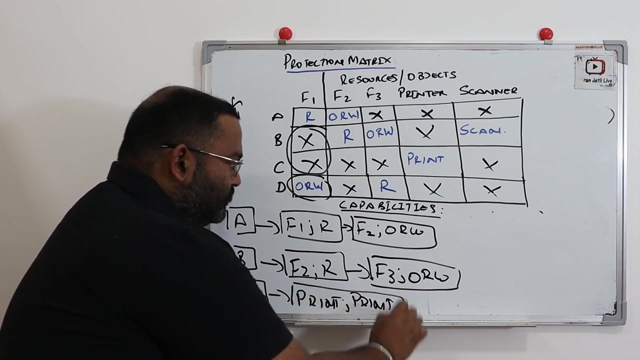 the next on F3, what it can do. it can own it, it can read it, it can write it and similarly I have process C. what process C can do? it can only access the source printer. it can use the printer and it can do print operation on that. and what?